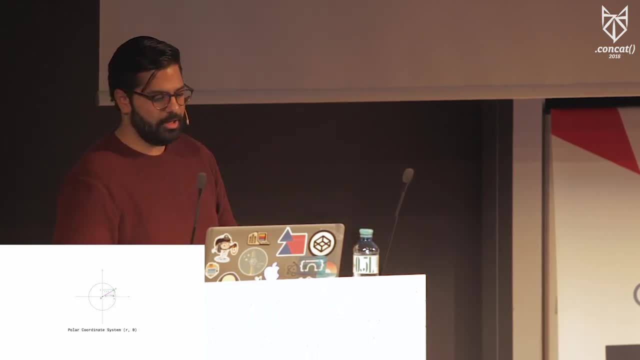 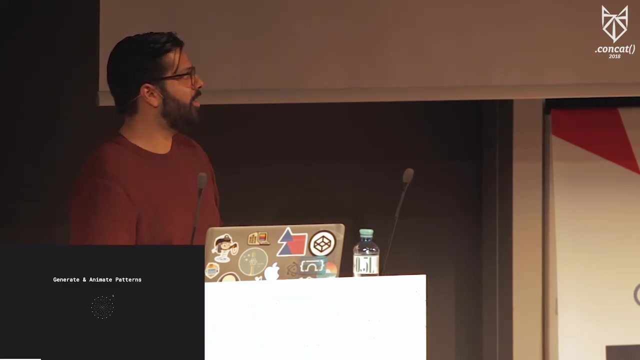 from the X axis. So why would you want to do this? In some cases, thinking about our geometry in terms of polar coordinates makes our life really easy. easy and allows us to do things which otherwise might be quite hard with Cartesian coordinates. An example of that is to build patterns such as these: These: 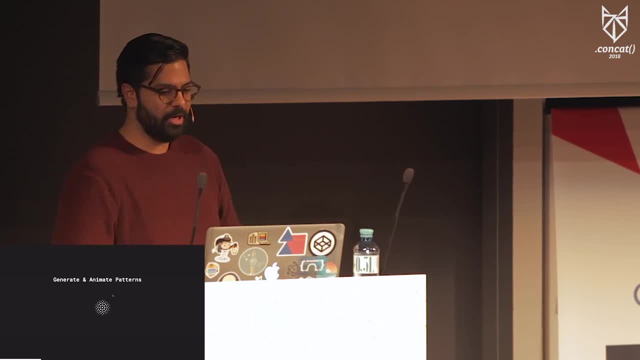 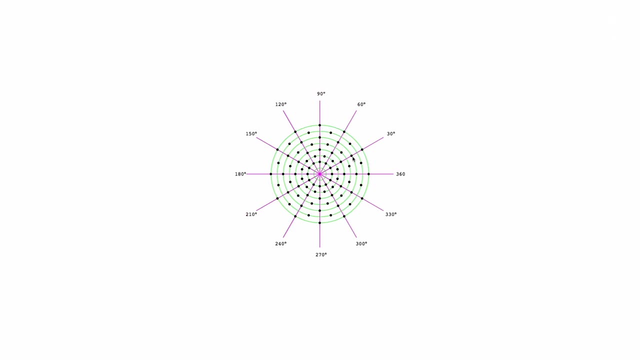 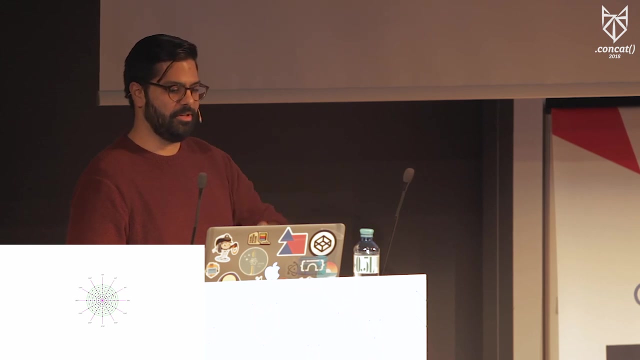 are known as polar patterns, and even animate them. So to do something like this you can use polar coordinates. and if I break down that shape, what it looks like is essentially it's layers of concentric circles, where on each circle you're placing these dots evenly around the circle so that at the outermost, 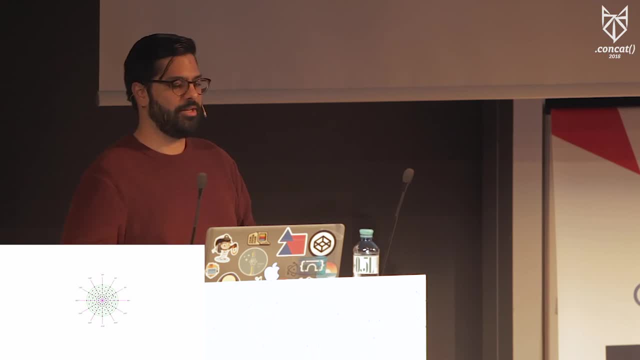 circle, you can set the value for the radius coordinate- sorry, the radius part of the coordinate- to be the same, and the only thing you're changing is the angle. So the first one starts at 0 degrees, then 30 degrees, 60 degrees and so on, and 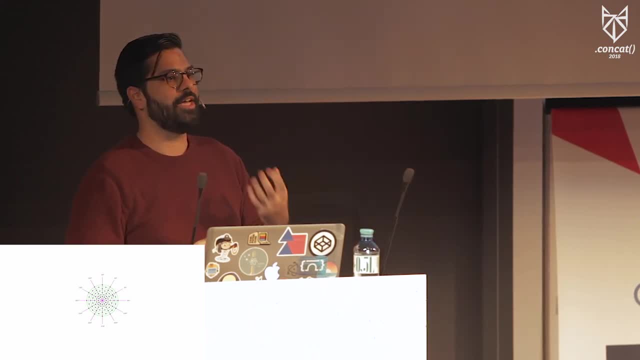 you can complete the whole circle And then to generate that pulsing motion, all you're doing is animating the, the radius value, and that causes the whole thing to scale down and scale back up, And this little trick allows you to do some really interesting work. 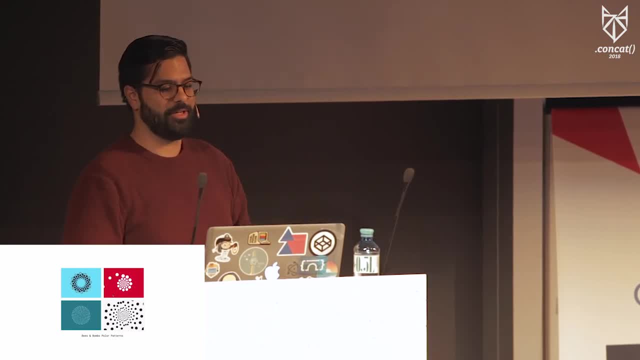 You can choose how you place things around on that circle. you can evenly space them out or offset them slightly. and when it comes to animation, you can choose to animate the radius, and that gives you the pulsing effect, or you can animate the, the theta value, which gives you more of the, the rotational effect. 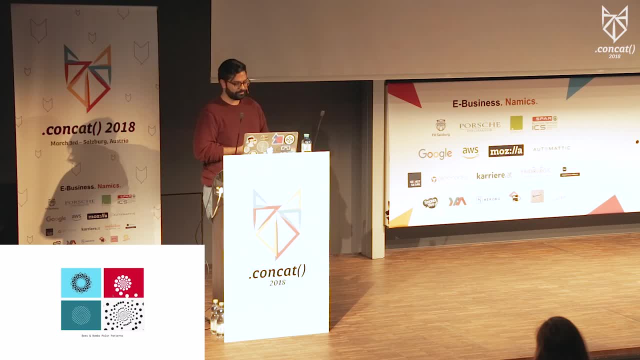 like the example in the bottom right hand corner. there We can also use polar coordinates to generate- dynamically generate polygons and specifically regular polygons. A regular polygon is just a a polygon where all of the sides have the same length and that particular shape has a special property, which is that the 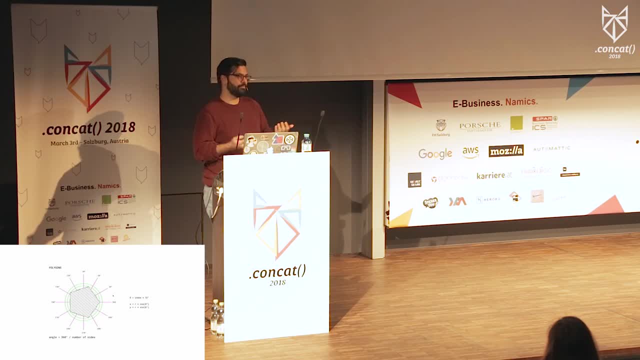 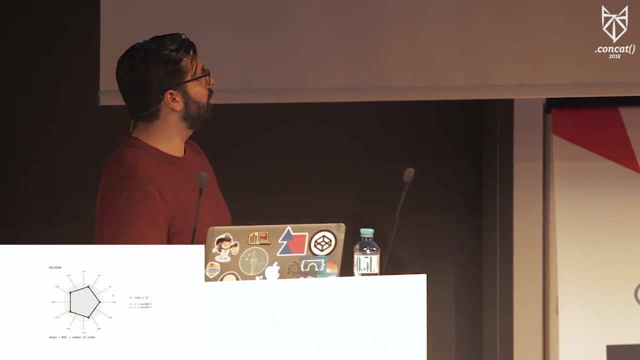 vertices, for for the polygon, are all on the same, are all essentially evenly spaced out on a circle. So much like the, the polar pattern I showed. the only difference is you end up joining them with a line and that that's what gives you the shape. So to locate the, the position of these vertices, the first one: 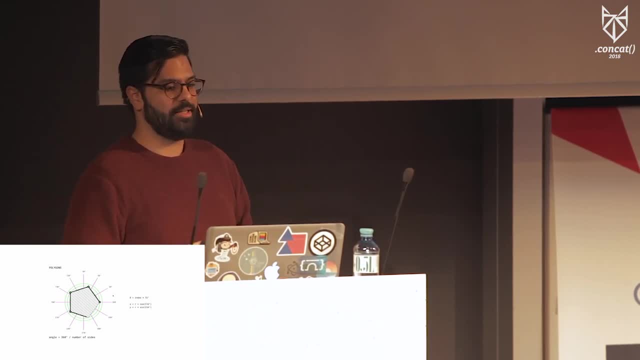 starts at theta of zero and that, and the second one starts at theta of a particular angle times the index, and that angle is the number of sides that the polygon has: 360 degrees divided by the number of sides that the polygon has. So the first index will be at zero times that angle. the second, 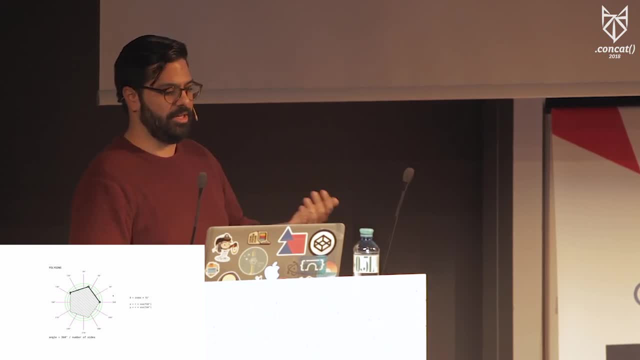 one at one times that angle, the third one at two times that angle and so on, And this allows us to generate the list of points of a regular polygon really easily. But then if you want to use them in an SVG path or canvas, you have to then. 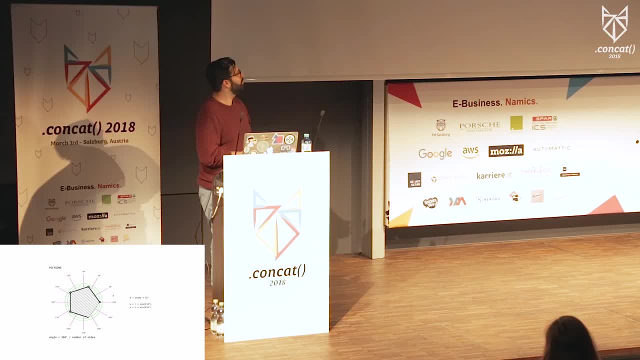 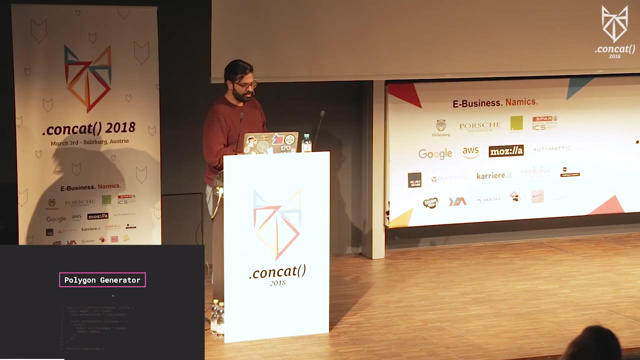 convert it back to Cartesian coordinates to actually render it onto the screen. And the way you can do that is by using this formula, where the X value of the coordinate is radius times cos of theta and the Y value is radius times sine of theta. So in JavaScript code that looks something like this: I have a little. 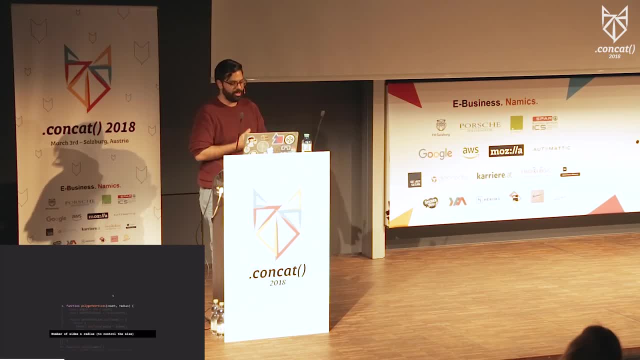 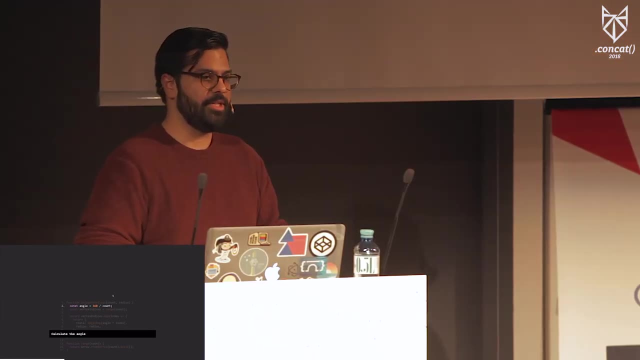 function here that is used to generate the vertices of a polygon. It takes in two variables: the number of sides that this polygon has and the radius, which sort of controls how big or small this polygon would be. And then the first thing we do is calculate the angle. 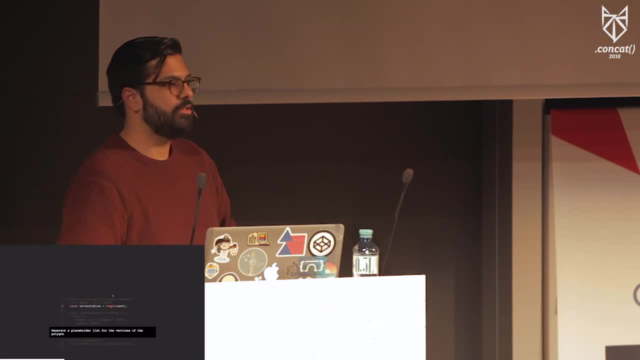 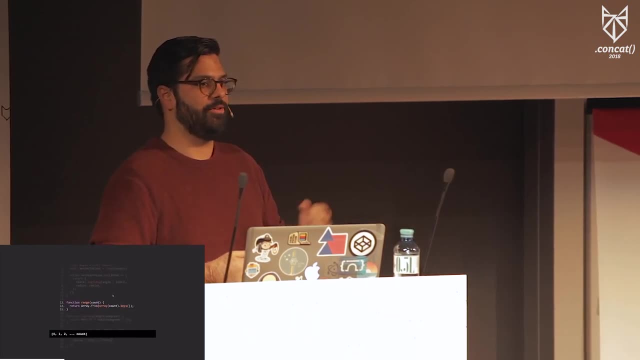 so 360 divided by the count. Then we create a placeholder for all of the vertices by using a little utility that spits out an array that has values 0,, 1,, 2,, all the way up to the number of sides that you specify. 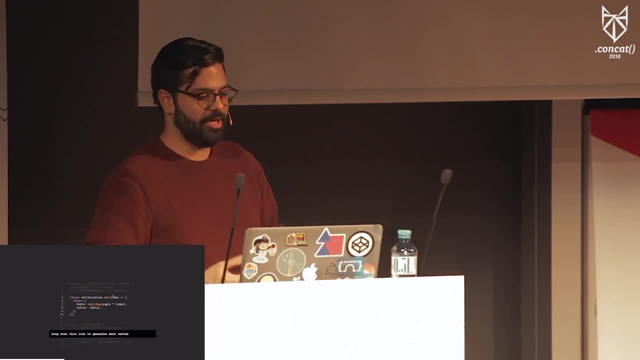 And then we map over this array to generate the coordinate where theta is angle times, the index of that vertex and the radius is whatever radius you pass in. And one thing to keep in mind here is, when it comes to humans, or especially me, thinking about angles in terms of degrees is really nice and makes my life easier, But when it 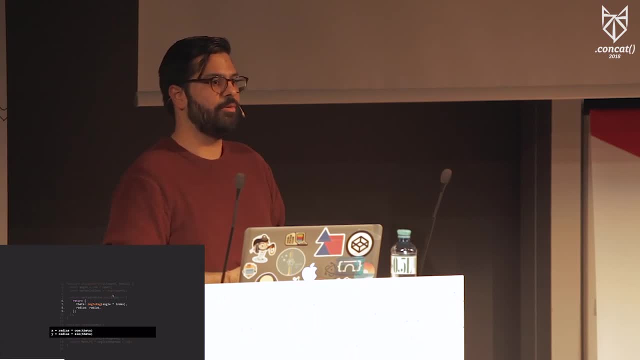 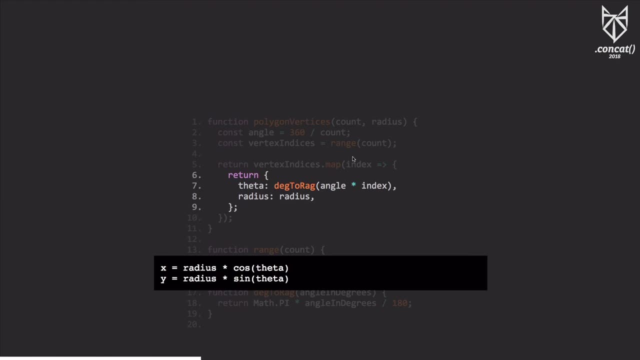 comes to writing code, pretty much every single time you're going to have to convert that value into radians. So that's what I'm doing here: I'm calculating the angle in terms of 360 degrees, but then converting it into radians and saving that as my value, And then once again to use this. 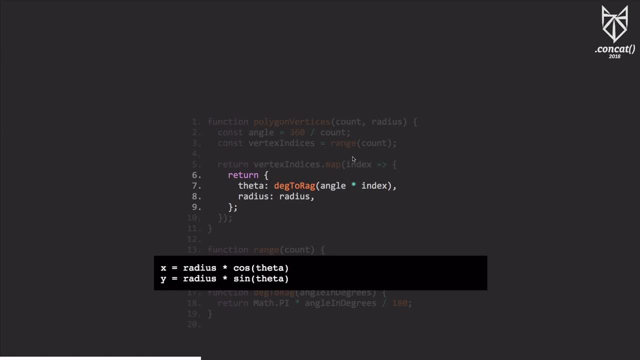 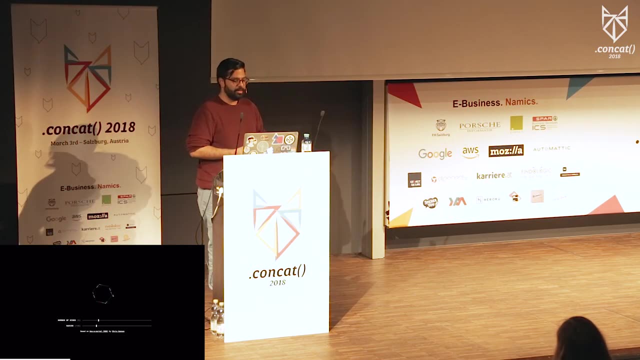 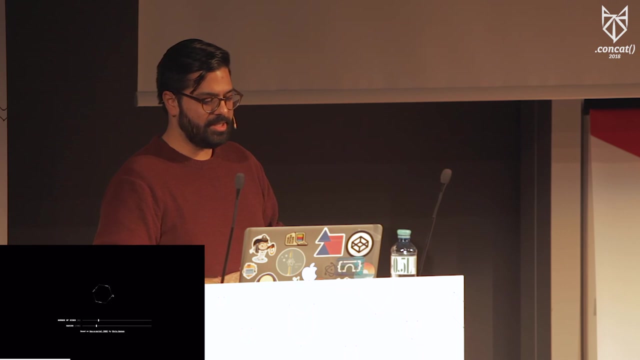 to render something, I can use the X and Y formula that I listed out there. So why would you want to do something like this? If you're generating your geometry dynamically, you can connect it to a user input. So in this case, I used an example. 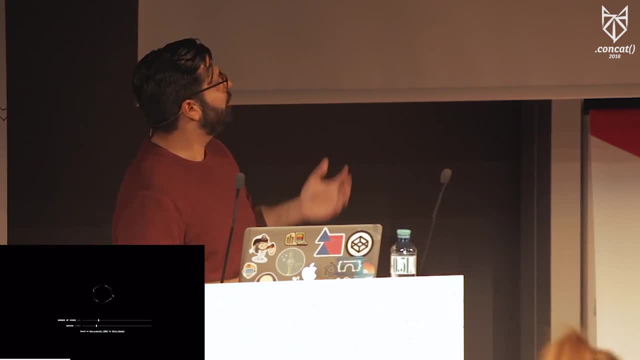 It was originally created by Chris Gannon. He created this really amazing hexagon that's being animated, And it was built out to be just a hexagon. So I modified this to replace it with dynamically generated geometry And wired it up to a couple of sliders. So with 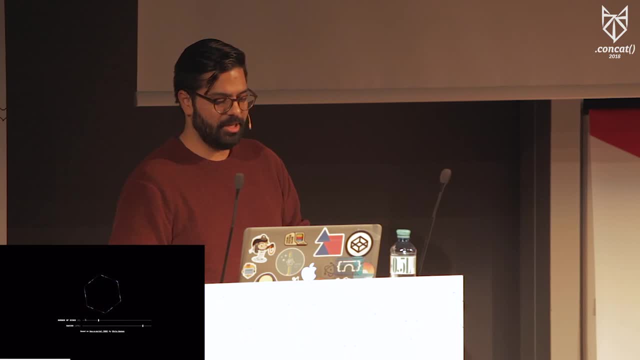 the radius slider I can sort of control how big or small the shape is, And then, with the other slider that controls the number of sides, I can sort of change what shape is being generated. So it's the same CSS code That's being used to render the animation, But I'm applying it to different geometry. 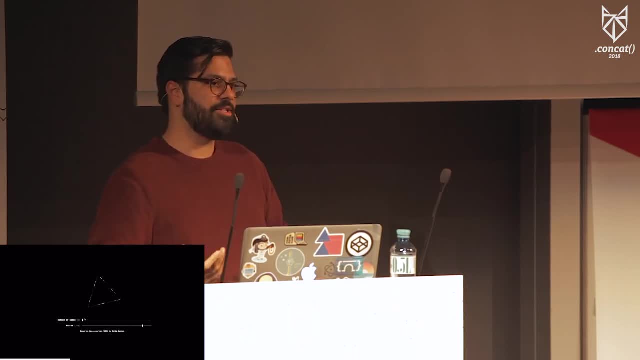 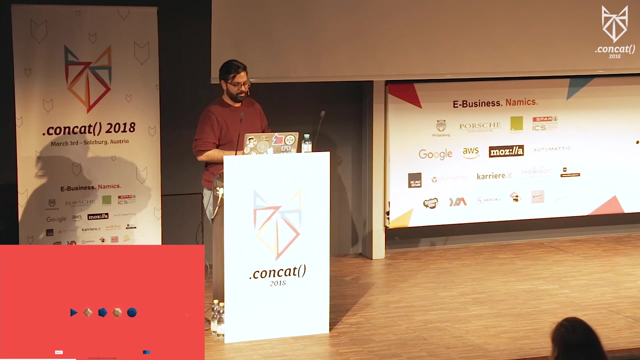 on the page, And you don't have to connect this to sliders. You can use any kind of data or any kind of user input to add a little bit of dynamic animation to your page. Another example is I made this demo a couple of years ago where, using the same polygon, 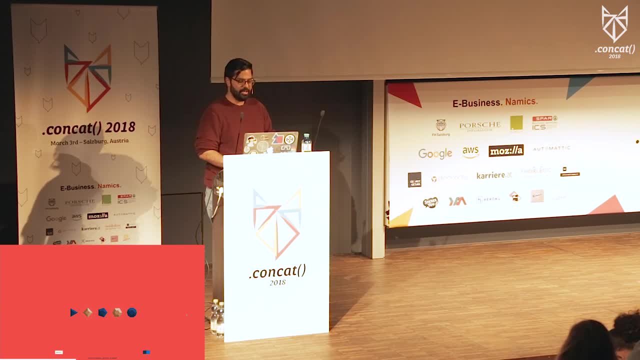 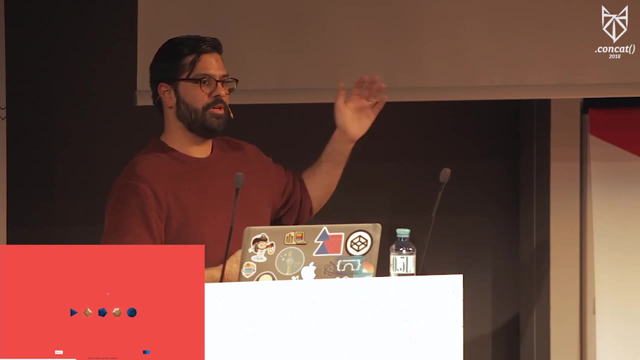 generator to spit out these shapes that look like sort of gems, And then wired it up to dynamic lighting, where the cursor controls where the location of lighting is. It's really basic toon shading style lighting And because this is built with SVG, sliced it up into different parts And each part is just given a different color. 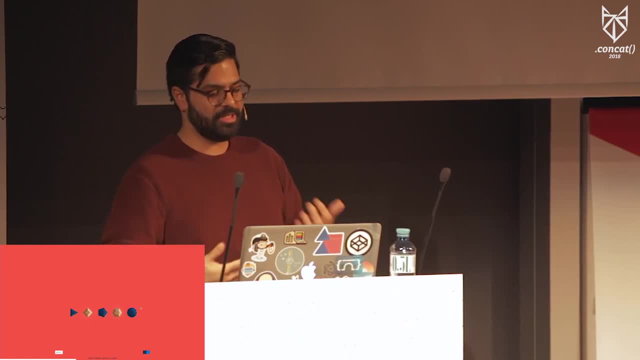 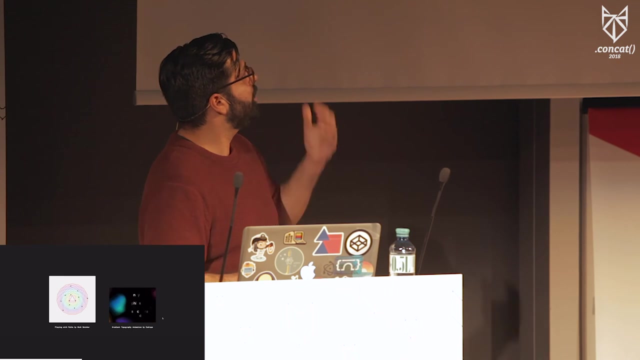 which simulates this lighting, And the reason I can do this is because I'm generating that geometry dynamically. I can sort of figure out and break it out into the different faces and color them accordingly. And some more examples that I've seen out on the Internet. Someone actually built out. 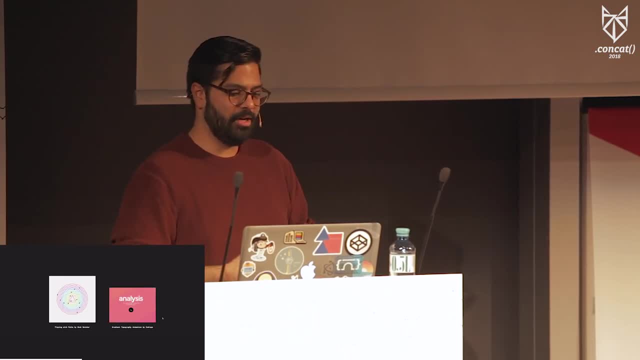 an animation loader using exactly the same polar coordinate pattern. And then Codrops had this fantastic article a few weeks ago that talked about building page transitions, and the shapes that they built out were these organic-looking blobs, And again they used polar coordinates to generate those shapes. 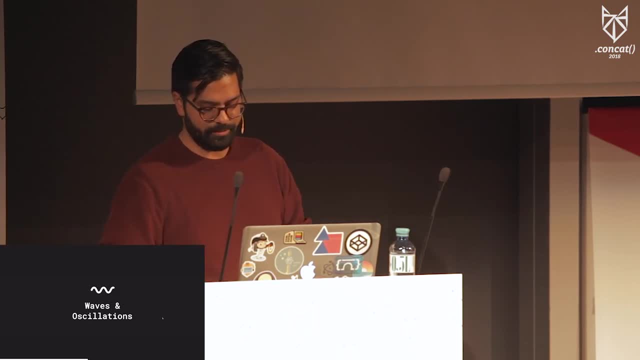 So, moving on to waves and oscillations, So there's this function that you're probably all aware of, called sine, that takes in an angle value and spits out a value that is somewhere between minus 1 and 1.. So, as you give it different angle values, it generates. 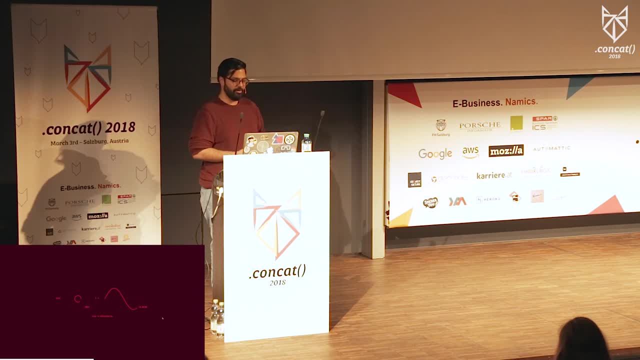 this wave-like pattern, Which looks quite boring but allows you to do some really interesting stuff. These are all GIFs created by an artist named Dave White, who also goes by the name Bees and Bomb. I really like his work, and one thing you'll notice is he uses this idea of 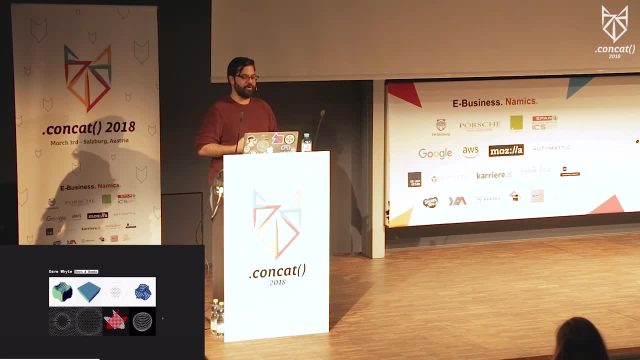 oscillations quite a lot in his work And he uses them to drive all kinds of things: The location of something, the scale of something, or even the scale, size, color and so on. So let's look at how we would do something like this. 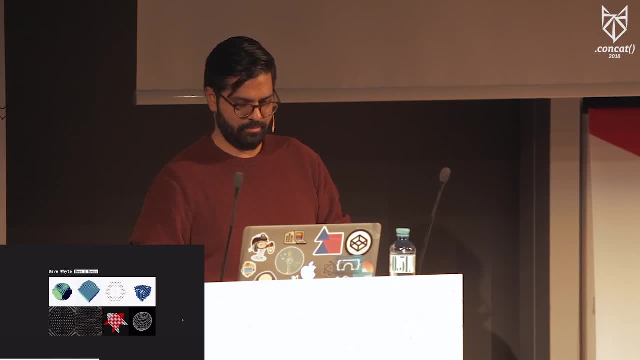 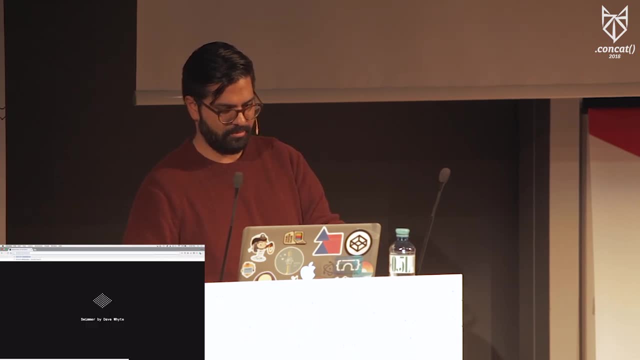 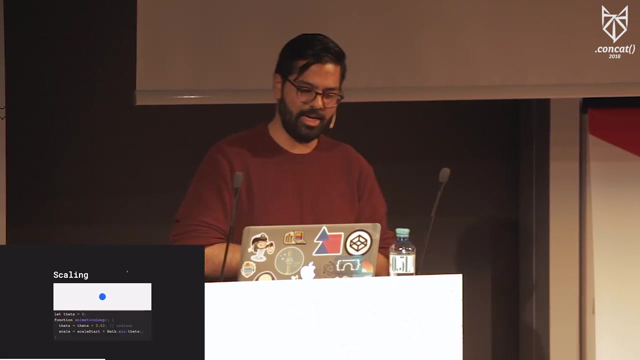 So here I have a little setup that demonstrates how to use sine to drive some kind of animation in an animation loop context. So I start by declaring a variable called theta- This is going to be the angle that we want- And I'm going to set it to zero, And then in my animation loop, I'm simply incrementing. 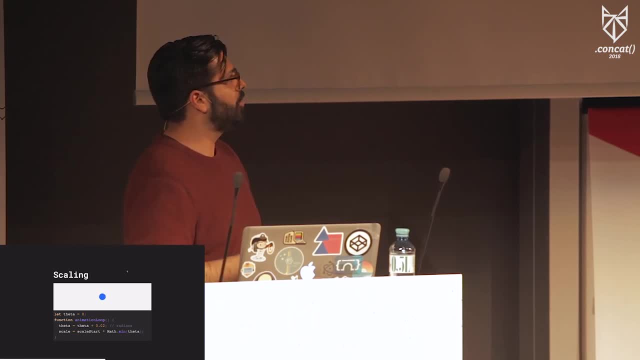 that theta with whatever value you choose. The larger that number will be, the faster the animation will be. The smaller that number, the slower the animation will be. And again, remember, this is in radians and not degrees, And then you can apply that theta to the sine. 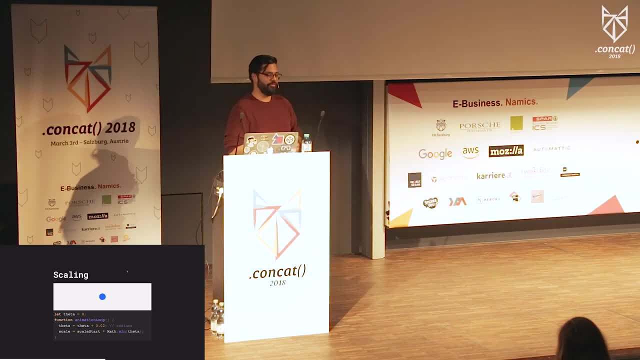 function in JavaScript and then use that to drive different parts of your animation. For example, if you're going to do something like this, you're going to want to have a number that's less than or equal to one. So if I multiply the output of that sine function, 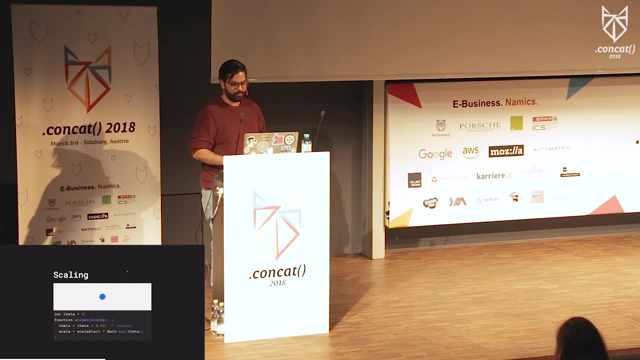 to the scale that gives you this pulsing effect. If I use that sine function to control the X coordinate, I can make something oscillate around a point. So in this case it's a slightly different format. You start with some basic. 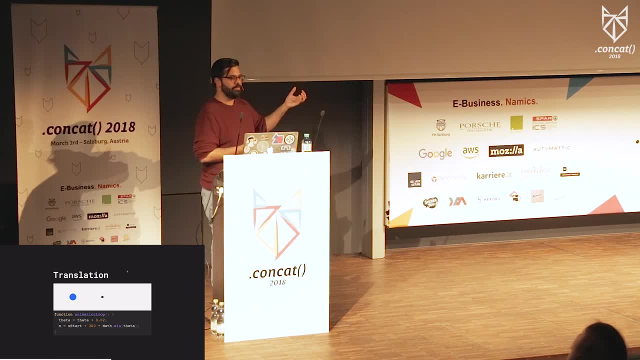 value, the base value of the X coordinate, that's the start value, And then to that you add the sine function times some amplitude, And in this case I'm picking 300 pixels, And that amplitude controls the pulse of the sine function. And then you can also add a. 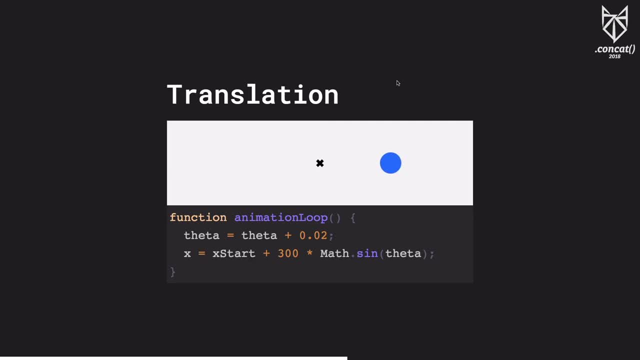 how far the ball is going to move around the X. So again, the larger the amplitude, the further it will go, the smaller, the closer it will stay. And then, lastly, you can also use it to rotate things about points. 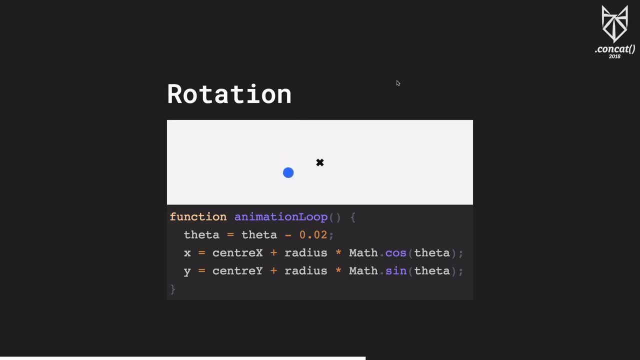 So, going back to that polar coordinates idea again, this time I'm using the same sine function- actually sine and cos- in this case they're both kind of related to each other- to calculate the X and Y coordinates. And since I want to rotate this about a point, 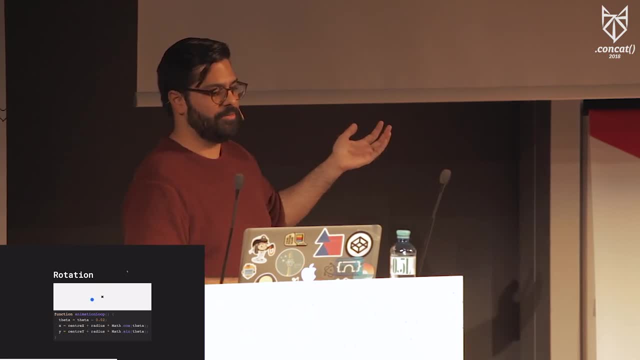 I also specify the initial values in terms of the center of rotation. So you're changing the place on the circle that this point appears by changing the theta value. but then you can translate into 2D space by adding center X or center Y to that value. 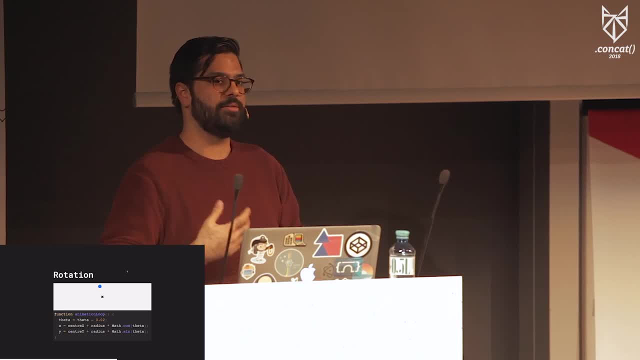 And this is sort of the starting point. You can combine sine and cos to create other kinds of motion which isn't just the static, not just the water, but one waveform motion. If you combine them, you can come up with some really, really interesting easings. 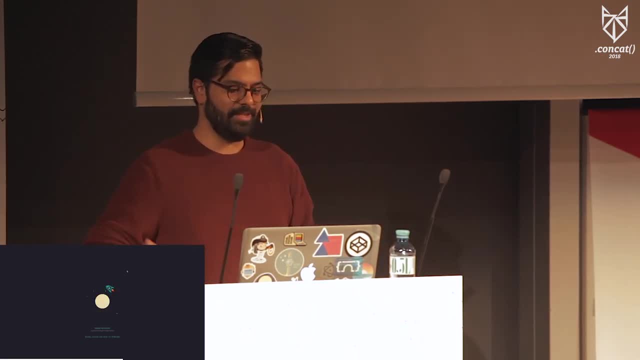 And this is sort of a more real-world example where someone used exactly that concept to rotate this spaceship around the moon. In this case it was done using JavaScript, but you can do the same thing with CSS animation if you want. So, going back to Dave White's work again, 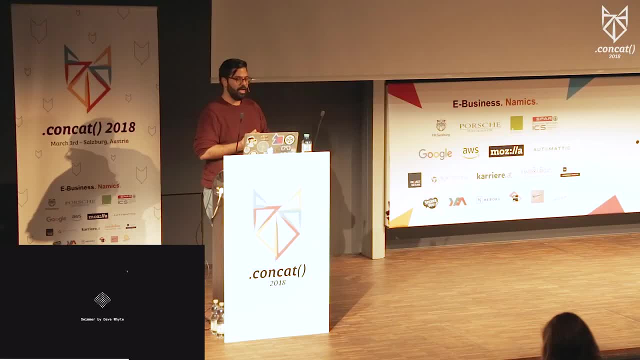 one thing you'll notice is in most of his work everything doesn't move at the same time. Things look a lot better, The animations look a lot more organic when things have a slightly delayed motion to them, So you can see each one of these circles. 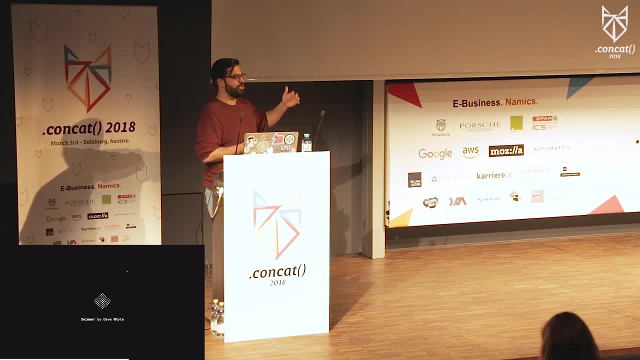 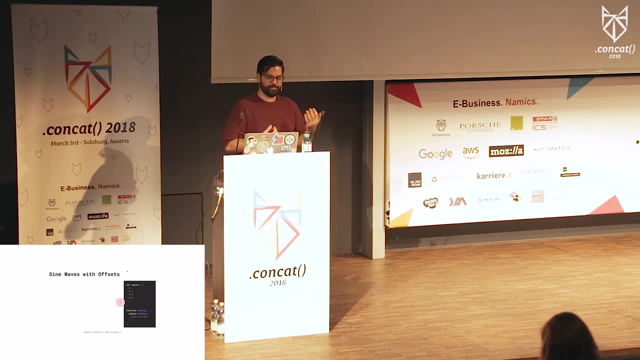 they're following the same path or the same amount of motion, but it just happens with offsets to each other. So the way you can do that is, let's say, start with this example of a ball which is bobbing up and down. 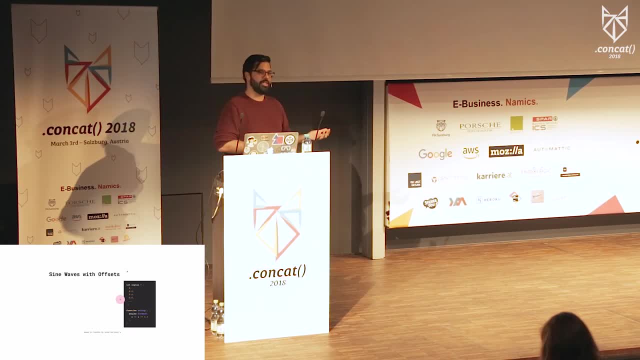 using that sine function And the initial value that we gave to this- the initial theta value was set to zero- You add another ball, but this time you gave it an initial value of 0.2, so there's a slight offset to it. 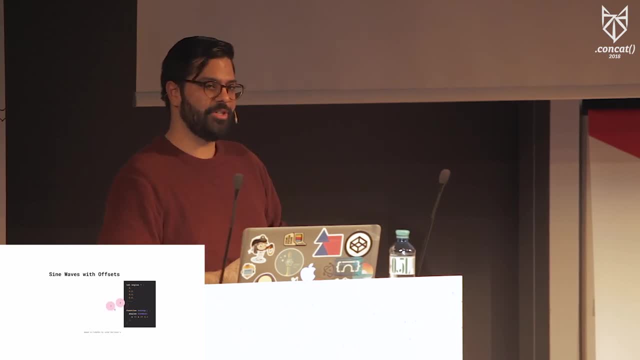 And you can see that already there's a slightly more interesting motion, or, in my opinion, slightly more interesting motion. And, as you can see, each time you add a ball and give it a slightly larger offset, you can create this nice wave-like pattern. 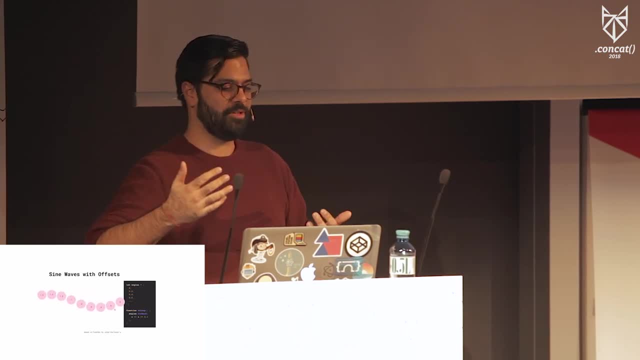 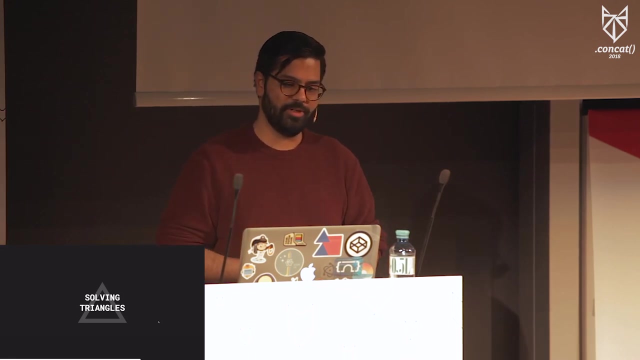 where each ball is moving in a wave-like motion, but then together they're creating a more complex motion. And then, of course, you can add layers to it to create even more interesting animations. And the last topic I want to cover today: 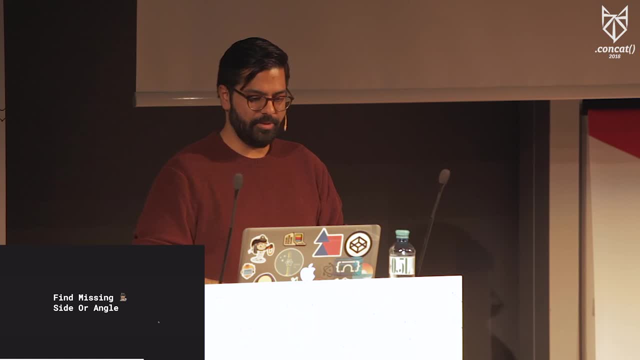 is solving triangles. So this is one of those things that once you learn about this, you see it everywhere. So I almost encountered this in just about every piece of animation I ever built, And really what this talks about is: you have some information about a triangle. 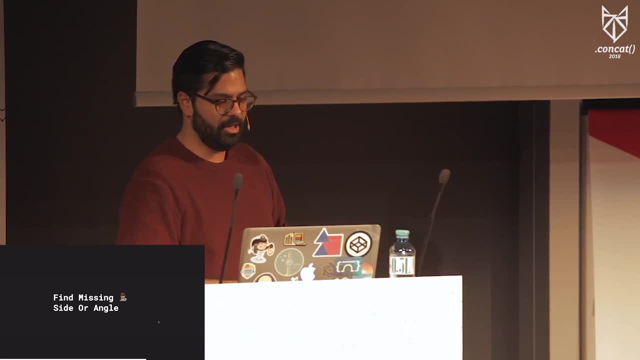 and you want to use that to figure out all the other properties of that triangle. So for example, that might be: you know the length of two sides and you want to figure out an angle, or you know two angles. 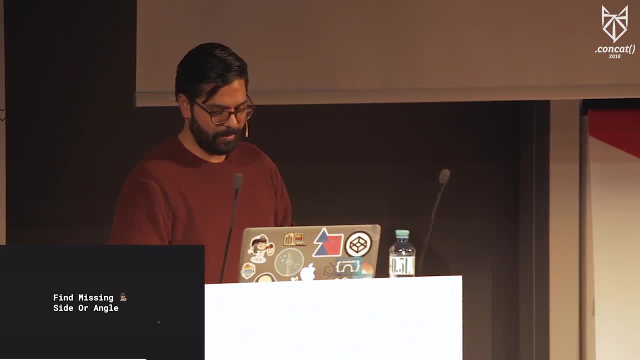 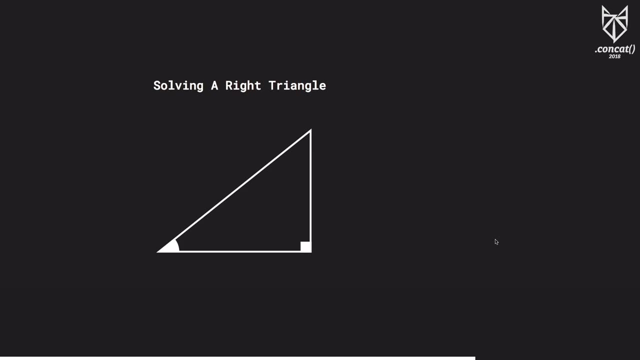 and you want to figure out the length of the sides. So I'll start with the most straightforward case, which is for a right triangle. So a right triangle is simply a triangle where one of the angles is 90 degrees. So in this case, 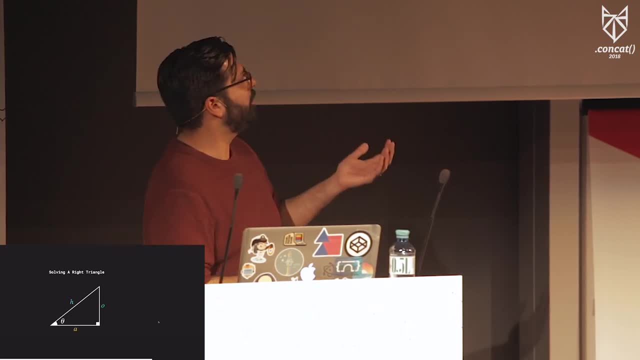 you might end up in that same scenario where you know the length of two of the sides and you want to figure out one of the angles, or vice versa. So for this I'm going to ask you to go back to high school. 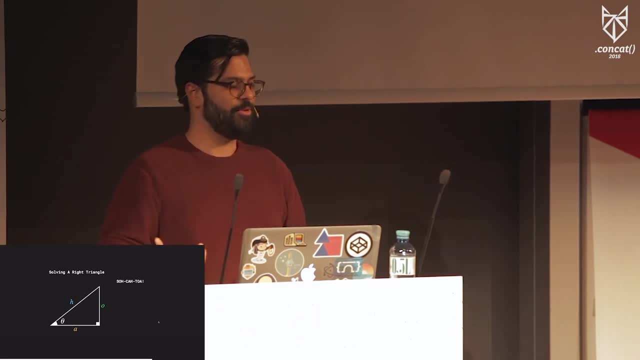 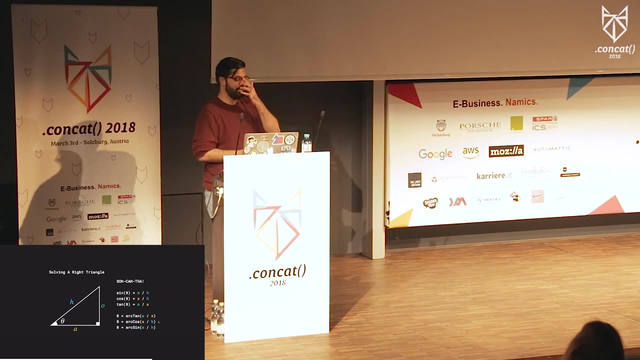 and you might remember this mnemonic device, SOHCAHTOA, from your math classes, especially the trigonometry part of it, And you might also remember these formulas that you encountered. That's exactly what you're going to be using here. 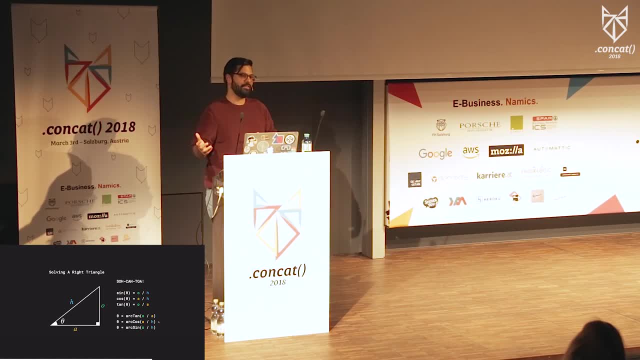 So back in high school, when you learned that math class and you were wondering why on earth would I ever need to know trigonometry, The answer is: animation. That's the only time you ever need it. So in this case, for example, 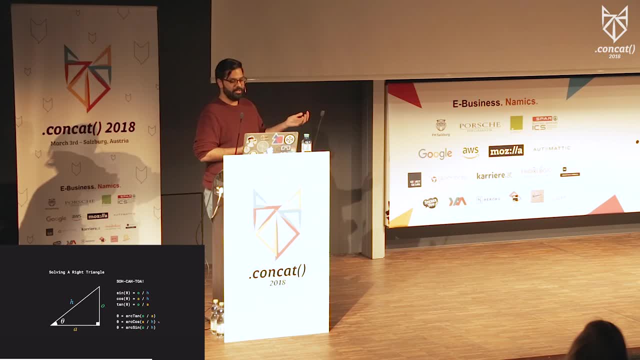 if we wanted to calculate the value of theta- and I knew two of the sides- I can use one of those formulas, for example the arc tangent or arc cosine or arc sine formulas, to figure out the value of theta. So let's look at some examples. 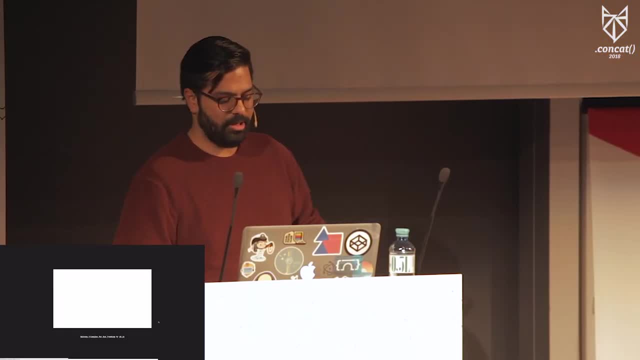 where this came in handy. This is an example from the p5.js website. They have a little eye-tracking animation, So these eyes follow the mouse cursor here, which is the blue dot that you see, And really the way this is done. 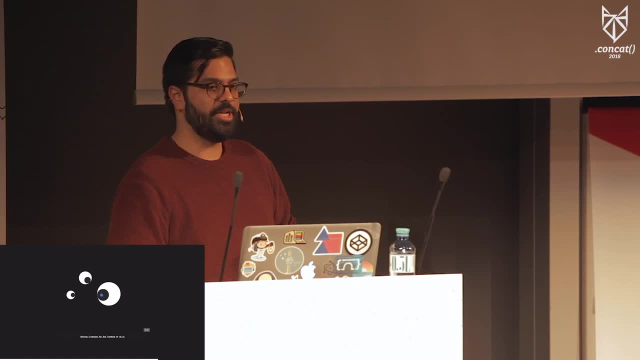 is the little black circle inside the white circle. you're changing the theta value. So, again going back to polar coordinates, all you're doing is you're changing the angle which decides where the circle ends up in the larger white circle. So this is sort of the triangle. 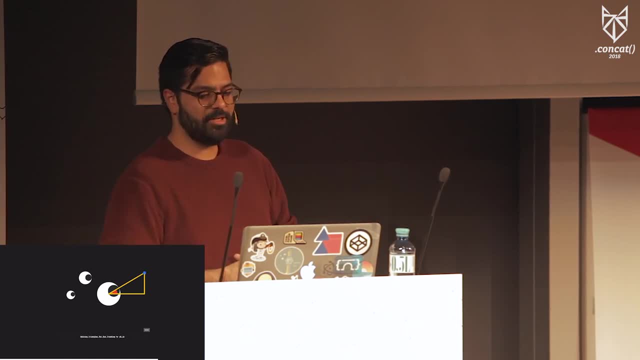 that we're forming here. Since I'm building this animation, I know the location of the mouse cursor and I know the location of the eye. So that means I know the horizontal distance between those two points. That's one side of the triangle. 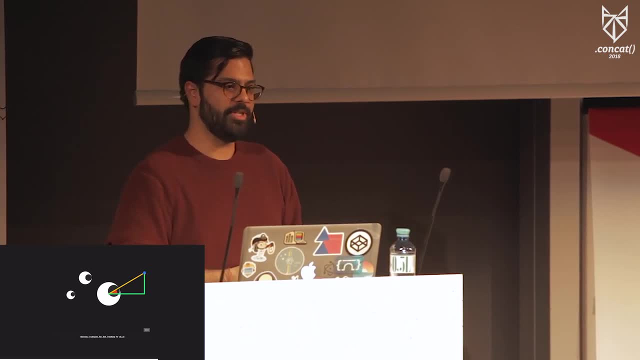 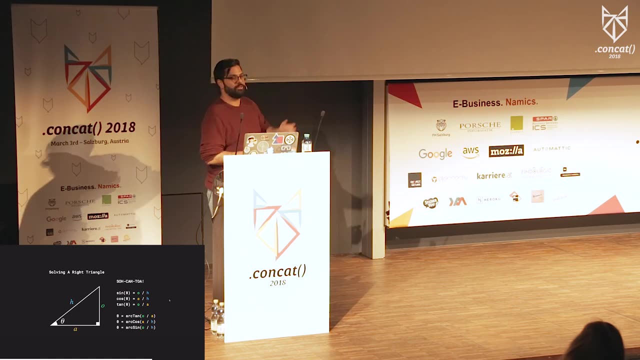 I also know the vertical distance between those two points. so that's the second side. So using that arc tangent formula, I can go back and calculate the theta value and then use that theta value to render out my animation. Another example: In this case, this is something. 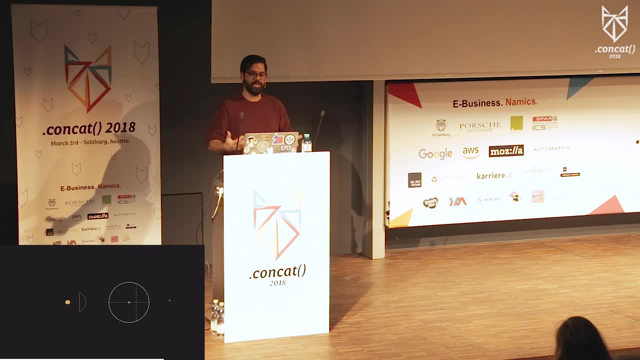 that I didn't really have to do in code, but just had to do it by hand or using a calculator before building out my animation. So to do this it's again using an SVG animation where the circle is breaking up into two parts. 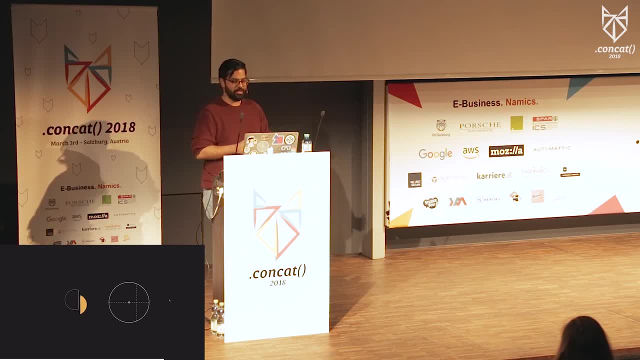 So I kind of know the ratio that I want to break the circle apart in. but to draw those two parts separately I have to use the SVG arc command, And to use the SVG arc command I need to know the exact location for those two points. 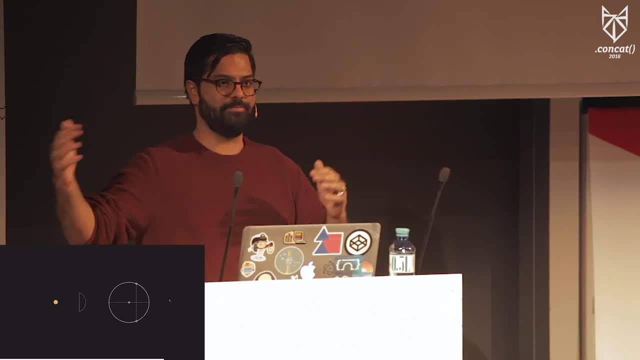 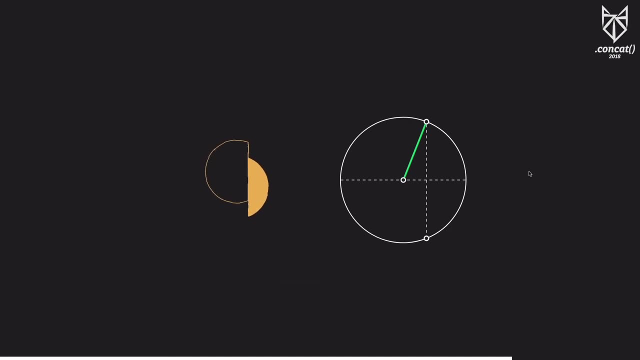 which is going to be the starting and the end point of the arc, and then simply choose whether I draw the larger side of the arc or the smaller side. So again, let's find that triangle. I know the distance between the center of the circle and those points. 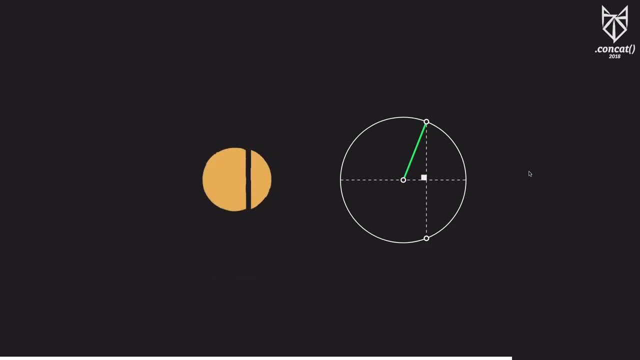 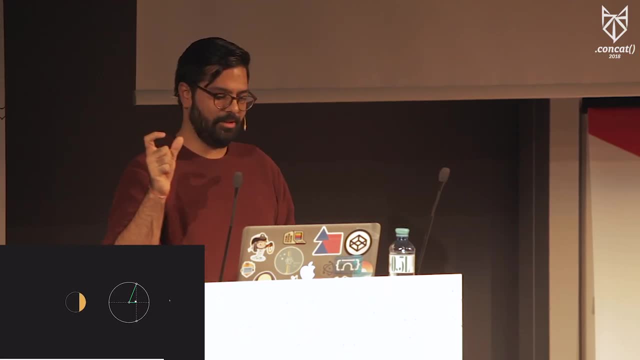 is just the radius of the circle. One of the angles is again 90 degrees, so we can go back to using those trigonometry formulas. And then, lastly, I knew the length of that little part there because I knew the ratios that I wanted to split up the circle in. 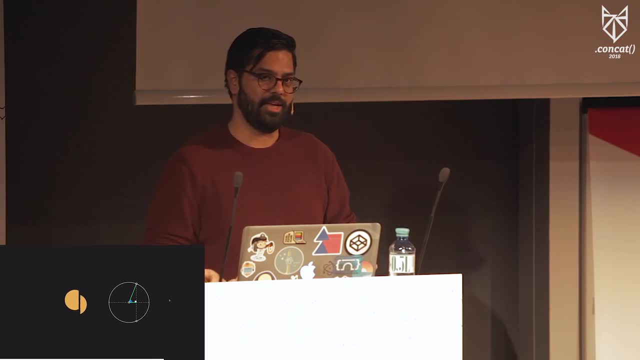 So, again using that information, I can calculate the angle and, going back to polar coordinates, use it to locate the two points and break up the circle into two arcs. So going beyond right triangles in a more generic use case where you're working with a triangle, 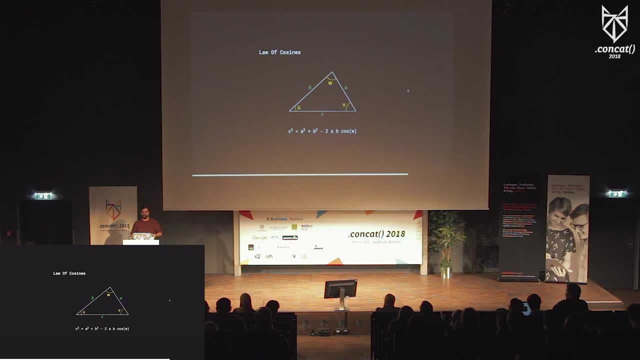 that's not a right triangle. in order to solve that triangle, you need slightly more information. So with a right triangle you just need two pieces of information. For all other kinds of triangles, you need at least three pieces of information. So whether that's three sides- 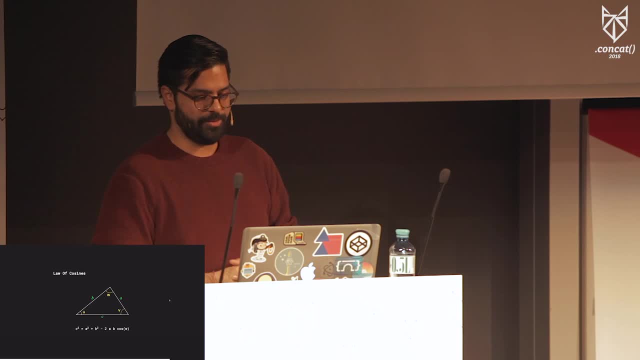 or two sides at an angle, or two angles at a side. any of those work And in that scenario you can use a formula called law of cosines. There's similarly something called line, which looks a lot similar. You can use either or. 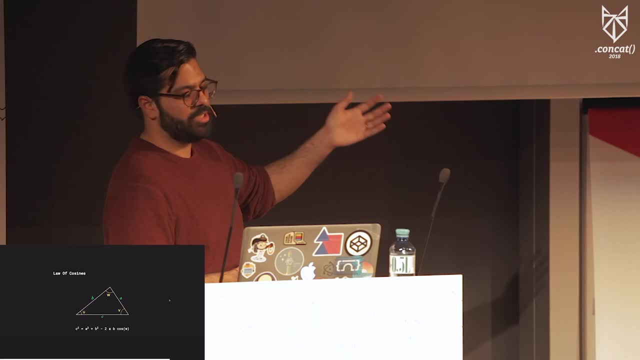 So in this case, you can pick and choose which sides that you have and which angles you have and apply it to this formula and figure out all of the other information of the triangle. So let's look at an example where I used this, So a few months ago. 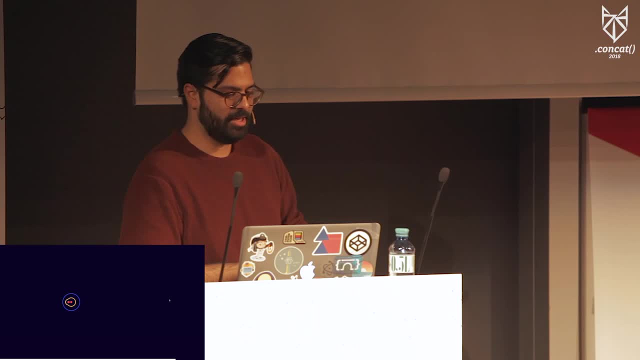 I built this animation, which essentially it's using a generative graphic concept known as metaballs, And there are much better ways to build metaballs, but for some reason I decided to build it with svgpath, which meant having to do a lot of math. 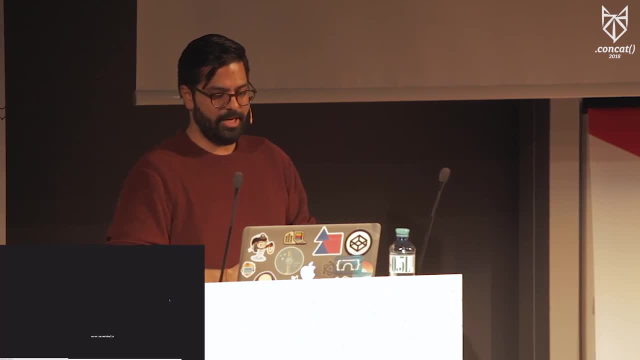 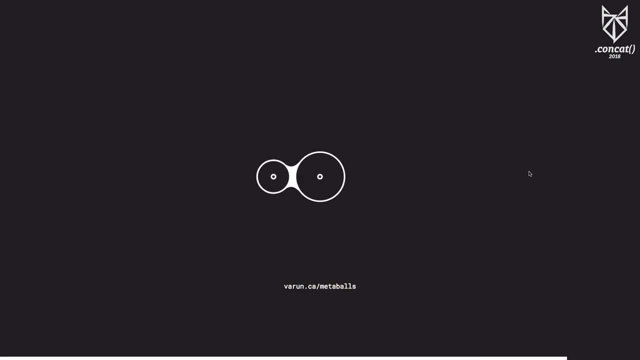 to figure out how to draw this, And what it comes down to is essentially there are two circles and then a little white connector that sort of allows you to mimic this blobby shape to it. I won't go into all the details of how. 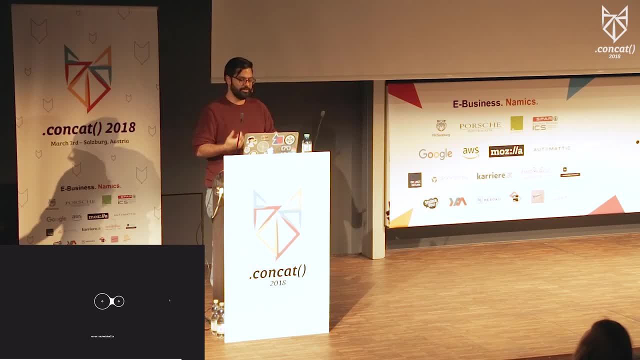 this happened. I have a link to a blog post down there that goes into that, But I want to focus on one specific part. So one of the steps in order to do this was to figure out these two angles, u1 and u2.. 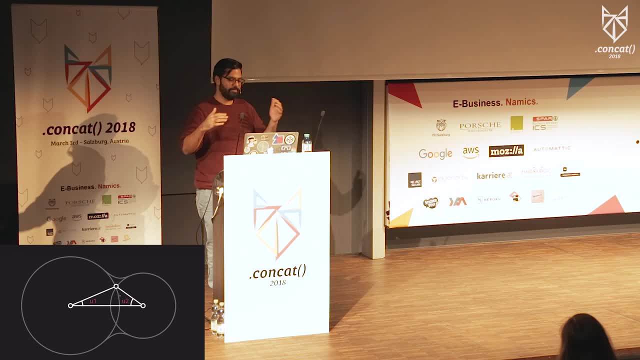 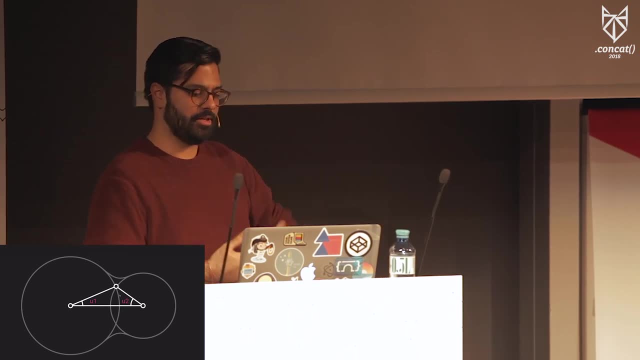 And these angles are formed by a triangle consisting of three points, which are the two centers of the circle and the point where the two circles intersect. So again I kind of know two sides, because they are the radius of the two circles.